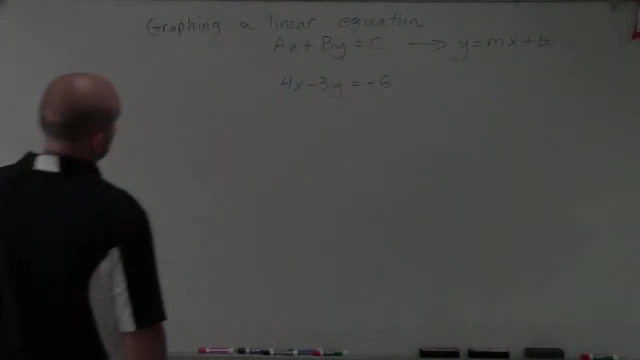 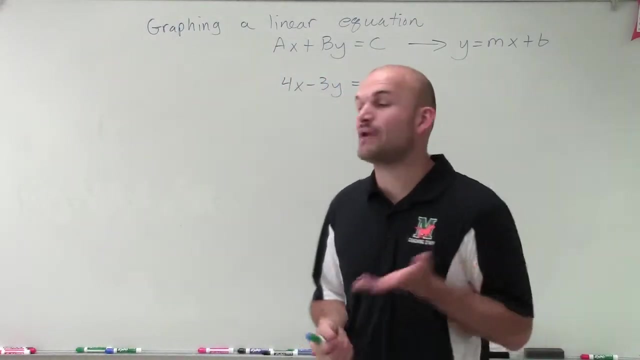 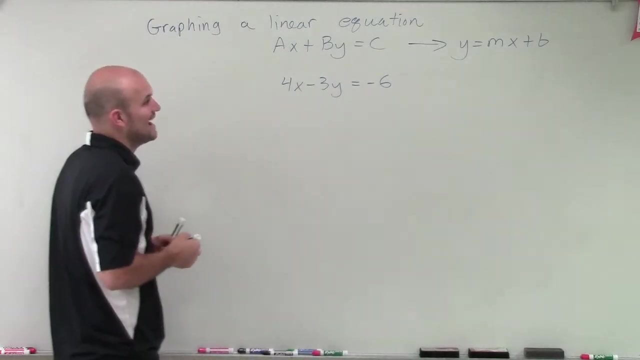 Welcome. So in this problem, this might be one where you might say, ah, I'm going to prefer to graph this in slope intercept form rather than trying to graph it in my x and y intercept form. And the reason being is because if I want to find the x intercept, the x intercept y equals 0.. 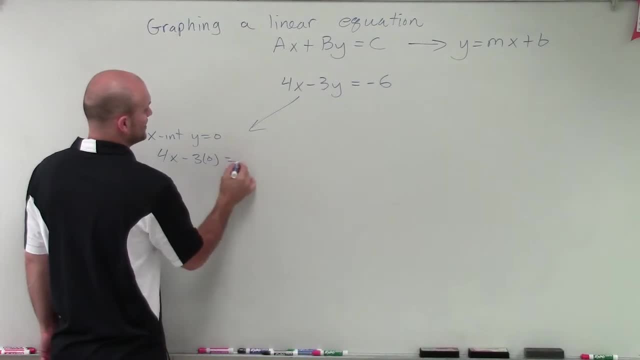 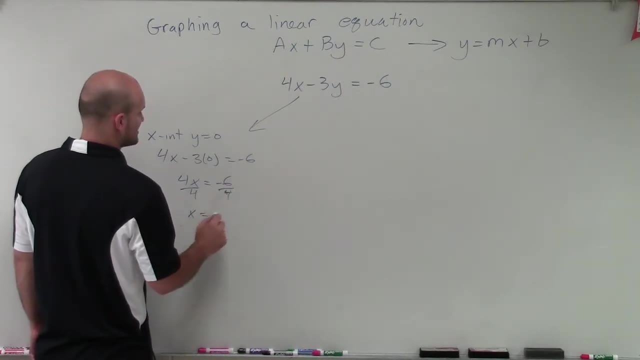 And I say: 4x minus 3 times 0 equals negative 6.. So therefore I have: 4x equals negative 6.. Divide by 4, divide by 4.. x is going to equal negative 3 halves. Now you could be like: ah, I just don't know how to graph this, or maybe it's confusing. 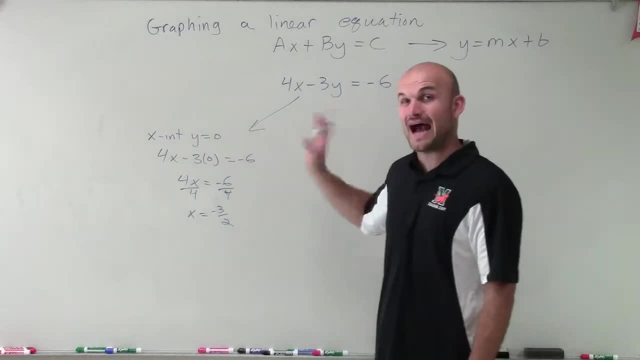 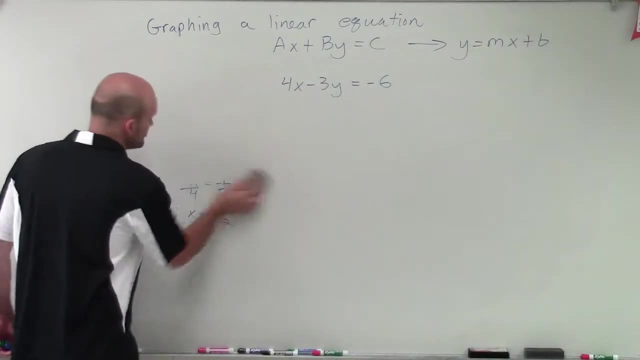 I mean, I showed videos on how to do this, But maybe you can see, with these fractions I don't want to be dealing with this. I understand slope intercept form, so I'd much rather just graph it that way. So that's why we want to make sure we can do both methods. 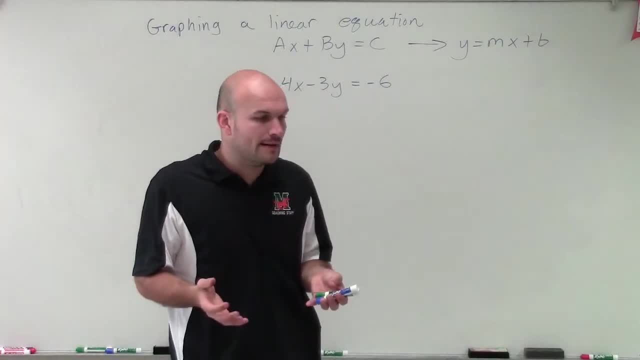 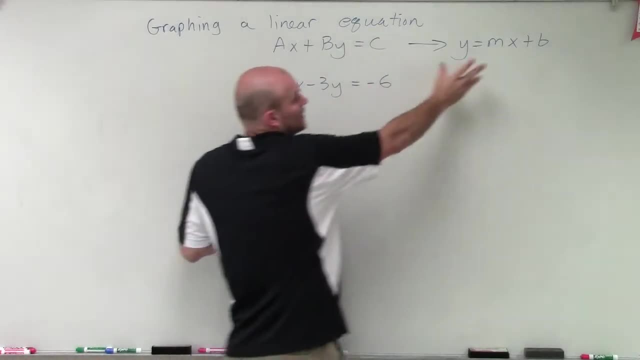 to determine on what equation is going to help us, what is going to be easiest to solve for either method. So what I'm going to do is I have an equation that's in my standard form and I'm going to convert it to my slope intercept form. 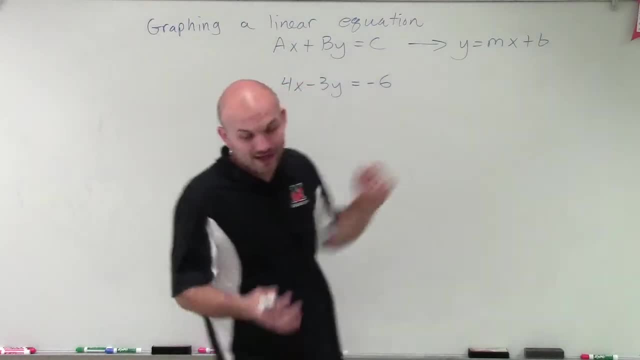 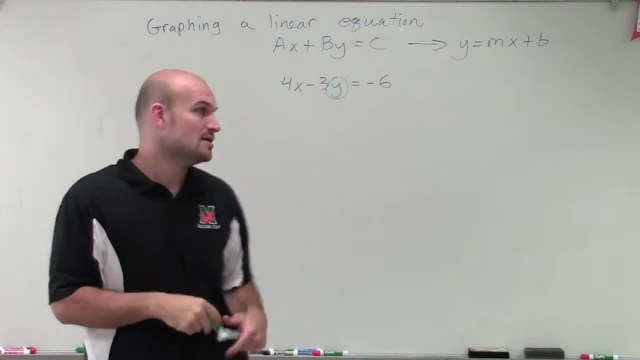 The main important thing I see with my slope intercept form is my y value is isolating. So what I need to do is I need to isolate this variable by using my inverse operations. So what we need to do is first, just like we were solving a two-step equation or any type, 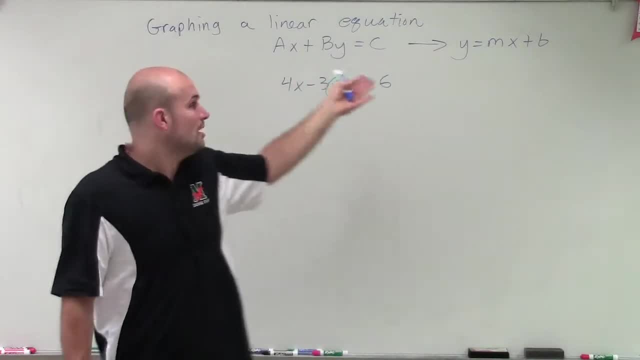 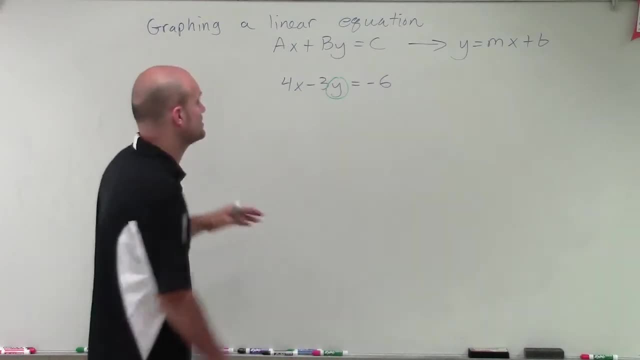 of equation. this one has two variables in it, so we call it a literal. But just when we're solving any type of these, we need to use our inverse operations, and we always undo addition and subtraction first. Now, since this 4x is positive, it's being added to my y. 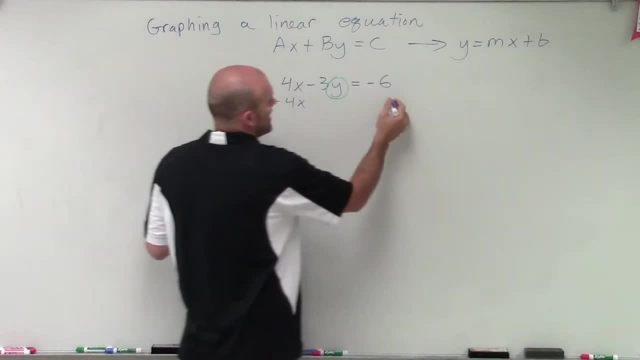 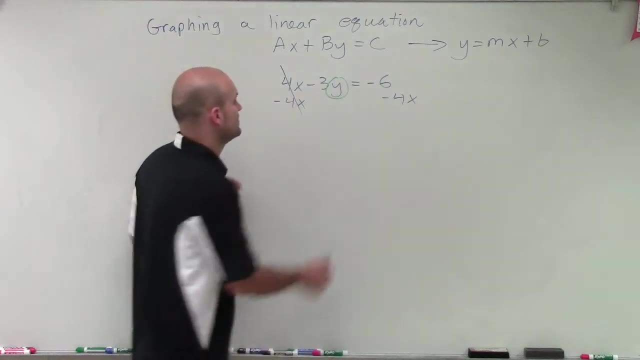 So to undo addition of 4x, I need to subtract 4x, And the reason why you can see, is well, if that's positive, then that's negative, That's going to undo, because then they'll add to 0.. 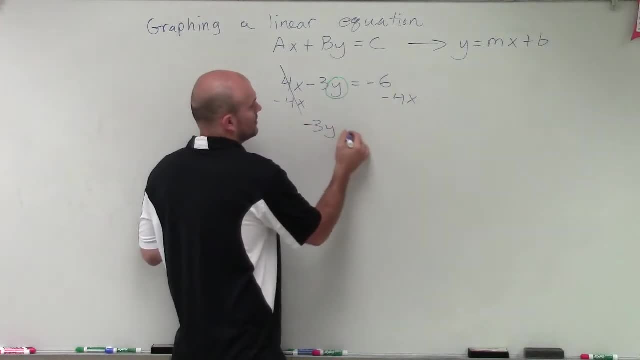 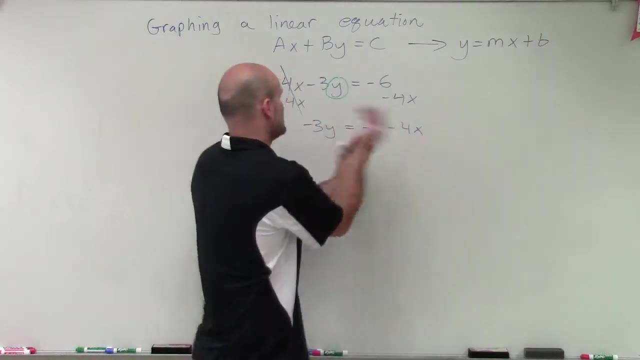 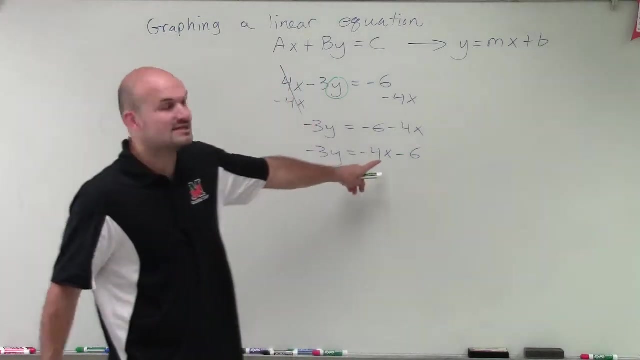 Now I'll still have a negative 3y is equal to a negative 6 minus 4x. However, remember we like to have the x in front of our constant, so I'm going to rearrange these And we cannot combine them because this: